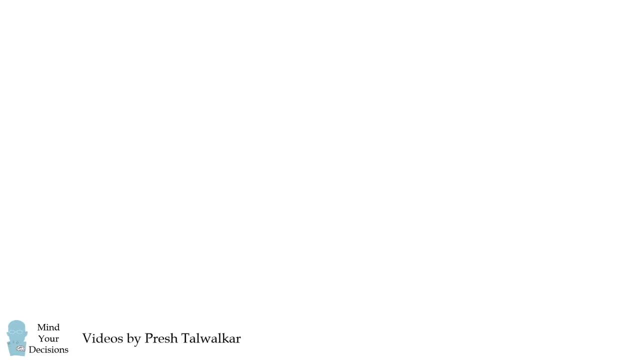 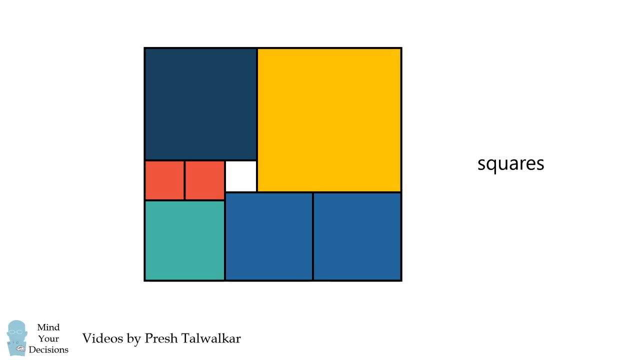 Mind your decisions. I'm Presh Talwalkar. A rectangle is divided into the following eight squares: If the smallest square in the center has a side length equal to one and an area equal to one, what is the area of the entire rectangle? 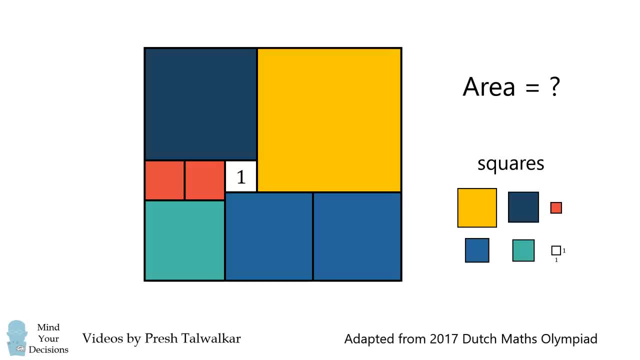 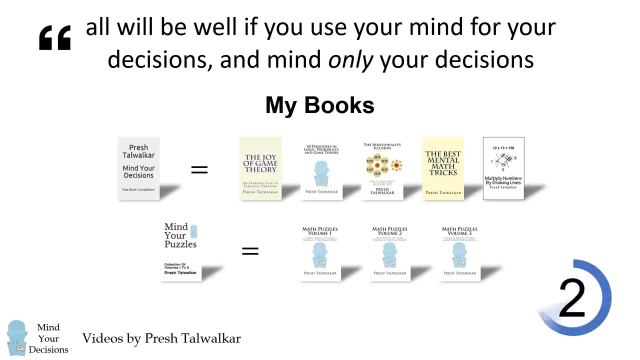 This question is adapted from one on the 2017 Dutch Maths Olympiad. Pause the video if you'd like to give this problem a try and, when you're ready, keep watching to learn how to solve this problem. So how can we solve this problem? 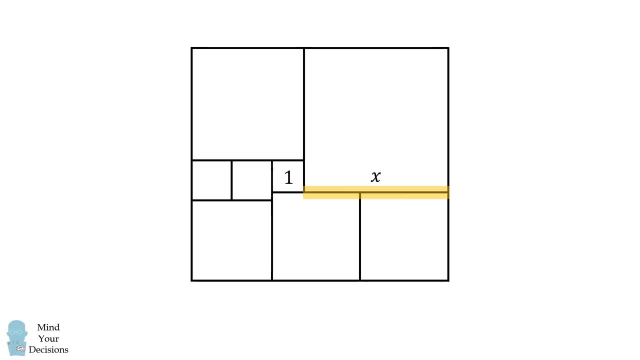 To get started, suppose the large square has a side length equal to x. We are then going to maneuver around this diagram like a maze and we're going to get another expression for the side length of this large square That will allow us to solve for x. then we can solve for the side lengths of the large rectangle and then we'll compute its area. 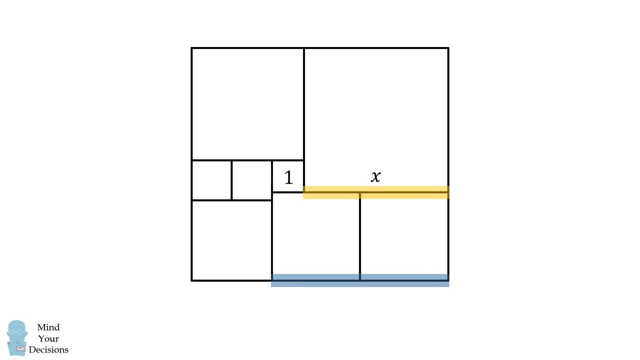 So let's get started. We will first compute this length, which is the sum of the two side lengths of these squares. It will be equal to 1 plus x. Each square will have a side length that's 1 half of that. 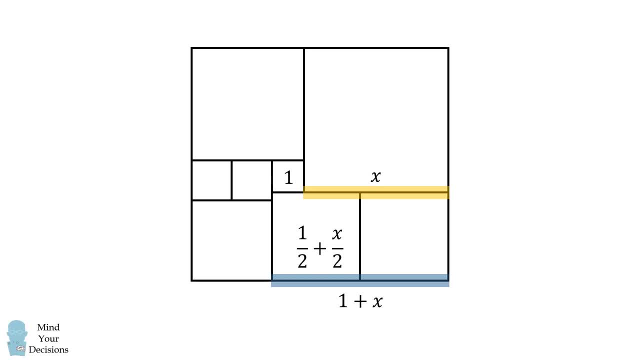 which will be equal to 1 half plus x over 2.. Let's now compute this distance. It'll be equal to the length of one of these squares plus 1, so it will be equal to 3 over 2, plus x over 2.. 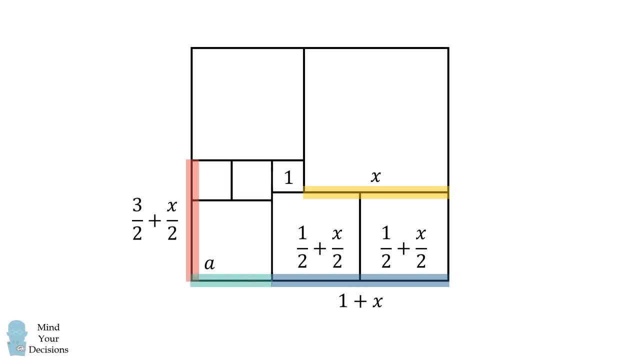 Now suppose this square has a side length equal to a. The two squares above it have a total length equal to a, which means each of them has a side length equal to a over 2.. Therefore, 3 over 2, multiplied by a is: 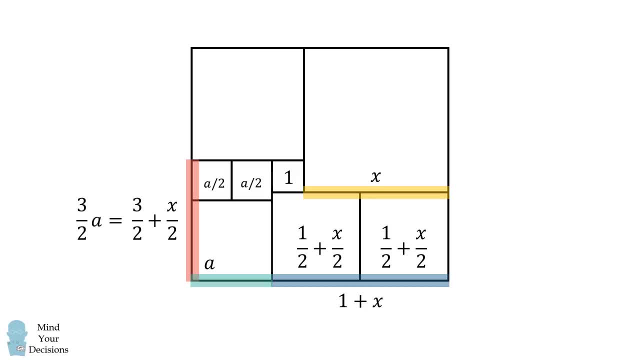 equal to 3 over 2 plus x over 2.. We can solve this equation for a to get that a is equal to 1 plus x over 3.. We can then compute this distance. It'll be equal to a plus 1, so it will be equal to 2 plus x over 3..